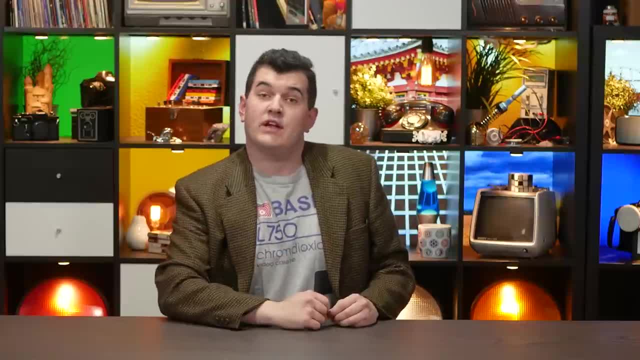 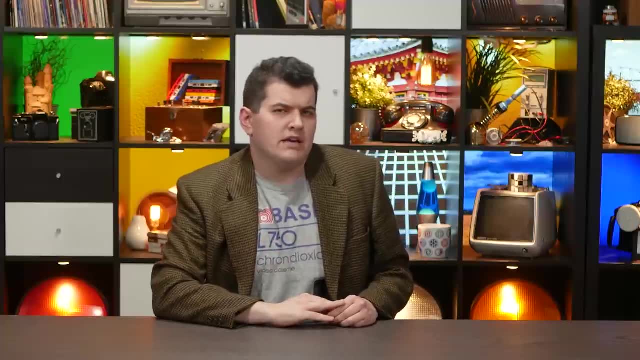 Have you ever seen a brown light? This may seem like a rather silly question, but it's pretty much the entire point of this video. So yeah, Now you've probably seen like a sign for a UPS store which is lit up and contains brown 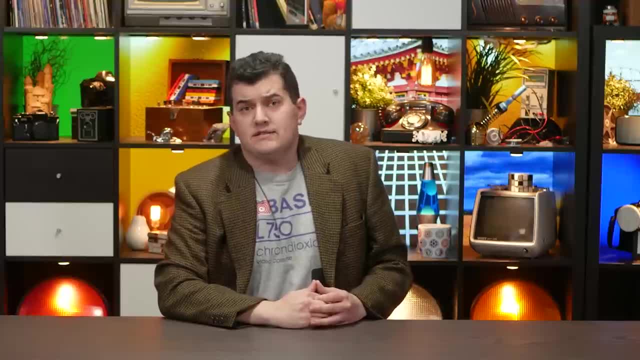 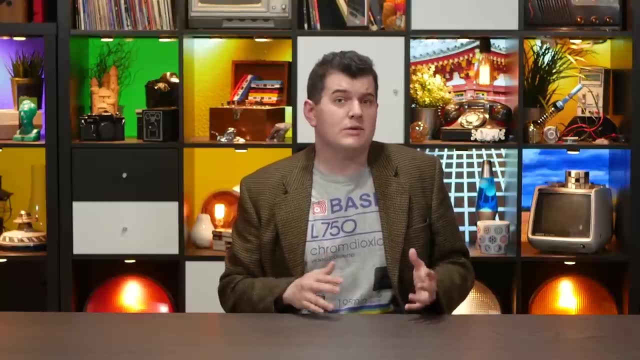 but there's a weird thing going on with that sign. It's not actually brown, It's orange. But darker Brown is an amazing color because it highlights how we perceive and describe the world. Our eyes are just fancy light detectors barely able to see three colors. 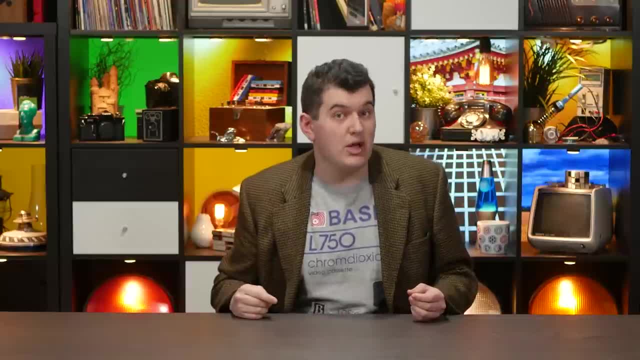 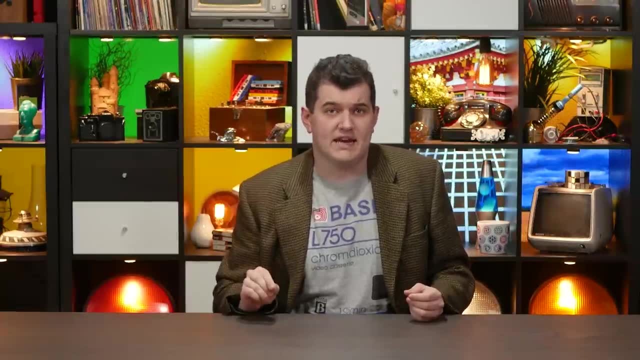 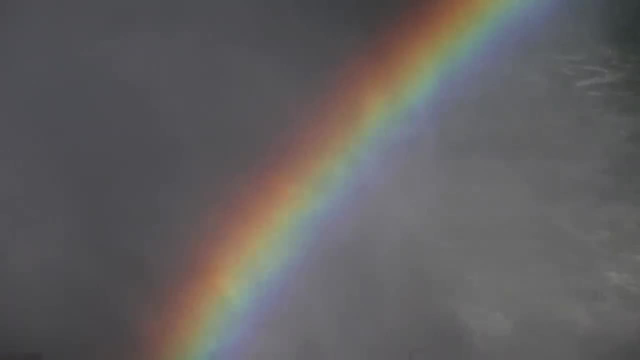 But our brains. They're pretty good at interpreting what the output from those light detectors means. And the fascinating thing about brown is that it's a color that exists due to context, not wavelength. Take a look at a rainbow. Rainbows are super helpful because they break out the visible light spectrum. 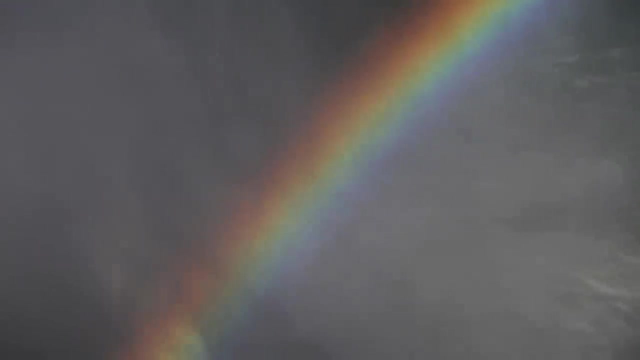 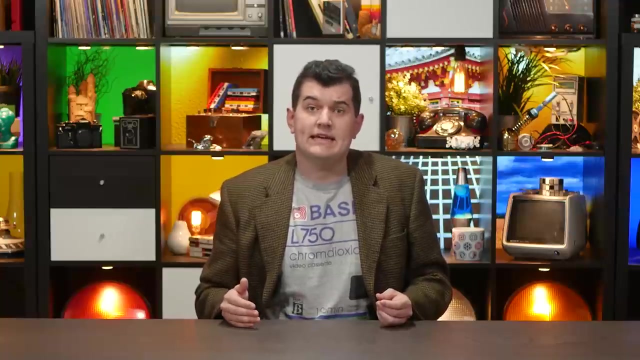 and show us the limits of what we can see. They're also super interesting because they exist only to humans. Well, They exist only to humans, They exist only to organisms that see invisible light, And they also kinda don't exist at all. 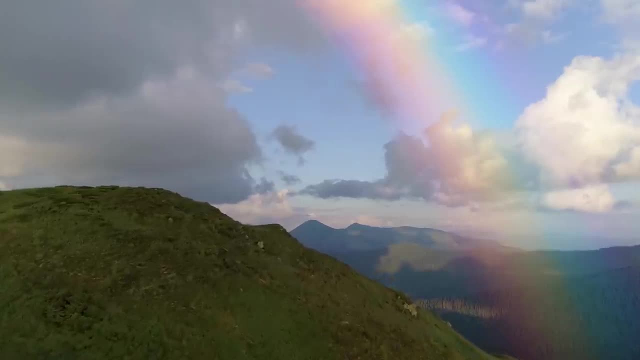 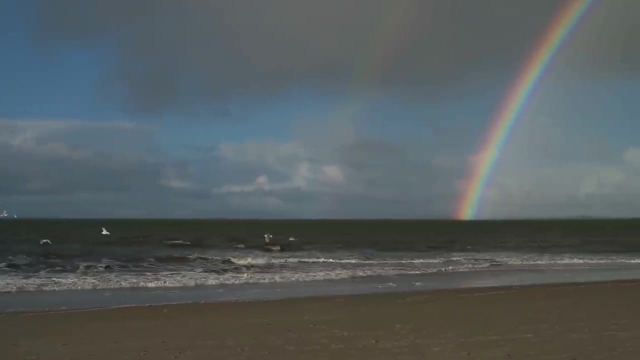 Rainbows aren't physical objects. they're just the result of weird things that happen when electromagnetic radiation gets diffracted and reflected through water droplets and observed from one location in space. Anyway, the important thing about rainbows is that they contain the color spectrum. 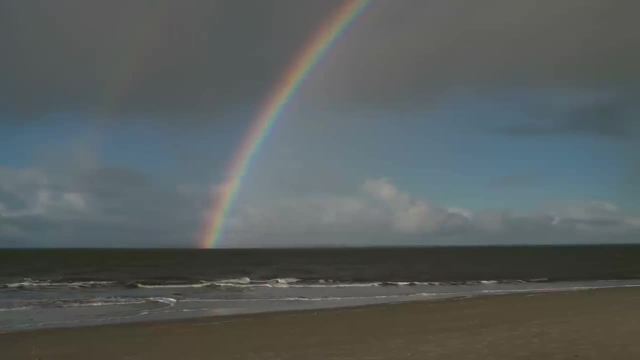 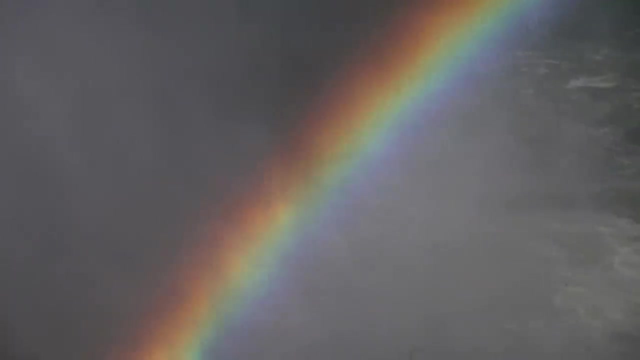 That's our friend Mr Biv Roy G. These are all the wavelengths of light that we can detect with our eyes and thus see. Now you may notice that brown's not in here. I suppose that's not too surprising. when's the last time you had a brown Skittle? 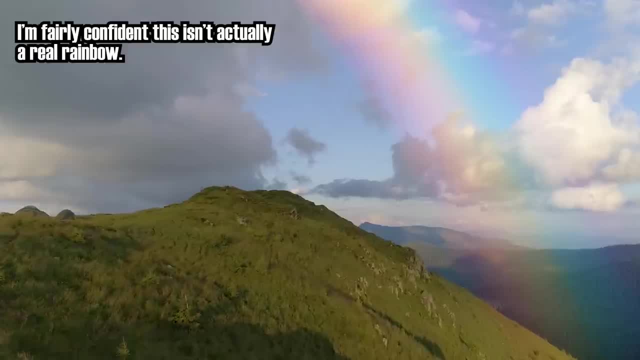 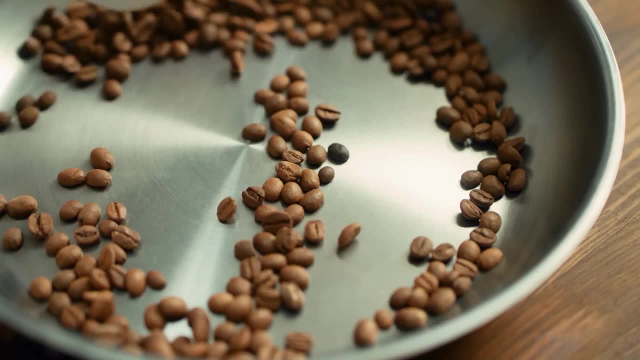 M&M's, though, Taste the brown. The fact that brown does not appear in the rainbow tells us that there is no such thing as brown light. Don't believe me. Well, I don't blame you. The screen you're looking at is showing you brown with light. 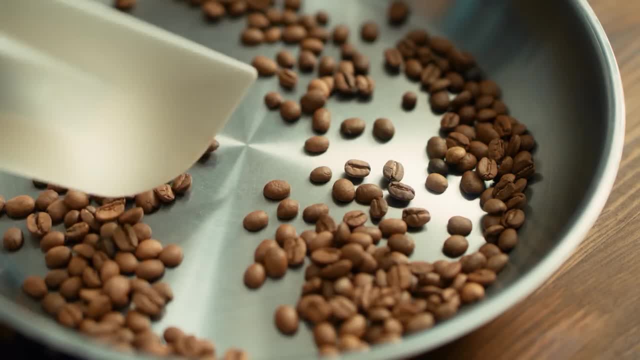 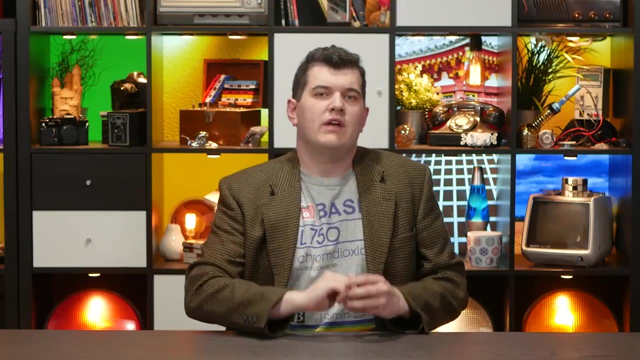 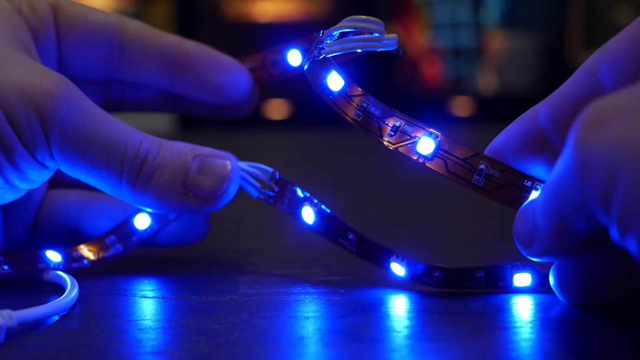 So how can there be no such thing as brown light when you're looking right at it? Well, in fact, this isn't brown, It's orange. with context, Let's play around with some RGB lights, shall we? I've gone with some LED tape light this time because I have more precise control over it. 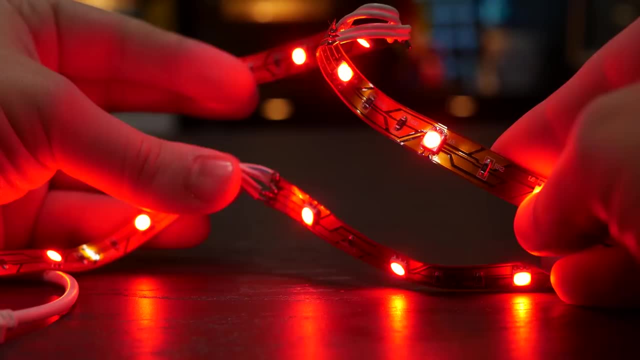 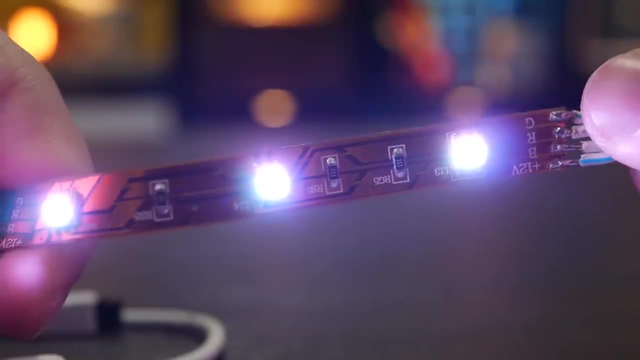 So quick refresher: the colors red, green and blue work together to create virtually all colors of light because they roughly correspond to the long, medium and short cone cells in your eyes. Mix the ratios up between these three colors and you can trick your brain into thinking. 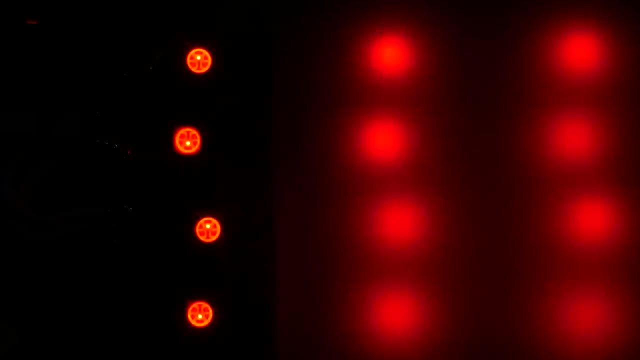 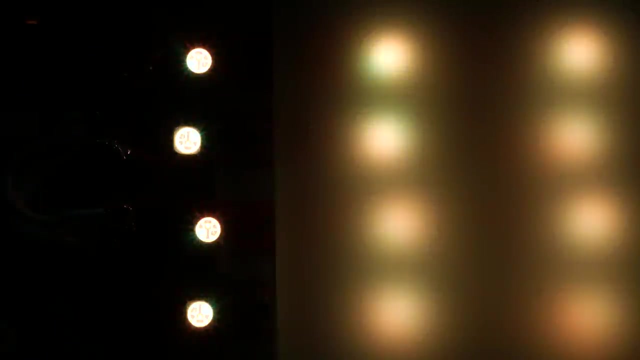 it's seeing just about any color at all, Red alone. Well, it's red. As we add green light, it shifts to orange, then yellow. Now, as we take away the red, it becomes a yellow-green and finally it's solidly green. 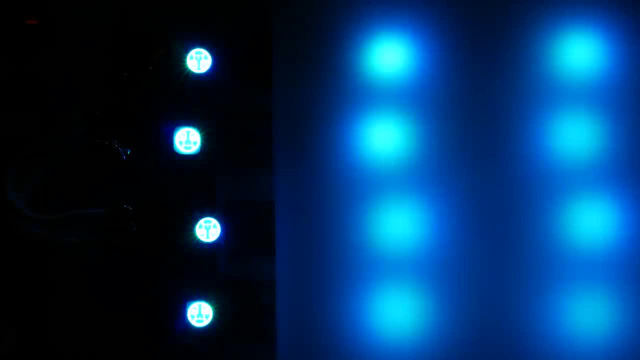 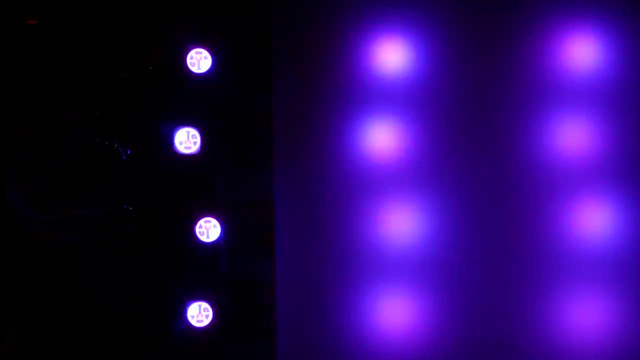 Then we add blue, and now it's shifting towards a blue-green and now a cyan before we start taking away the green and it heads into solid blue territory. Start to add red to this and you get a purplish color. keep going and we get magenta. 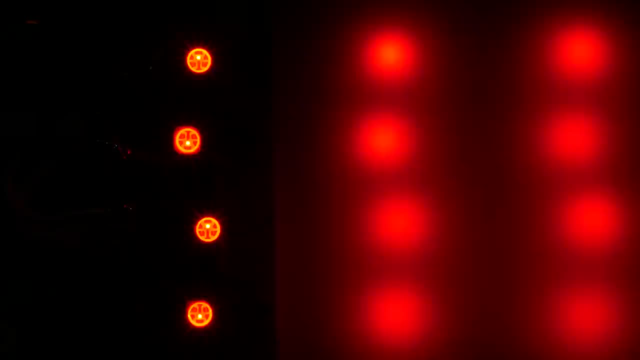 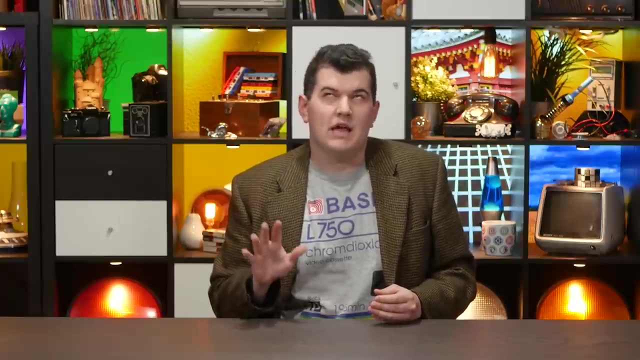 And finally, as we take the blue away, we start back at red. The only thing we've been messing with here is the hue At the Dewey or Louie, And hue exists on a circle. Well, sometimes There's a bunch of ways to represent color, but here let me show you my play button. 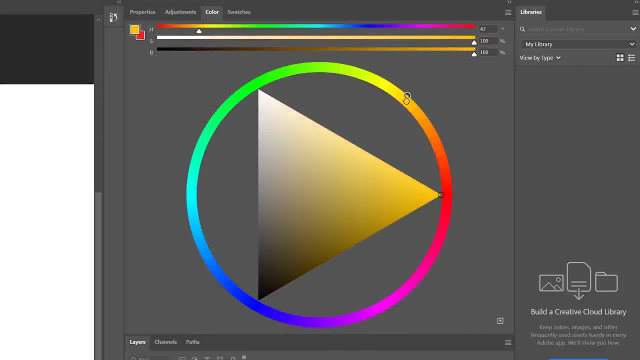 The outer ring contains all of the pure colors of light that we can produce in an RGB space. You'll notice that it follows the color spectrum, though violet is replaced with magenta and it bleeds back into red. In case you forgot, magenta is a weird color that our brains made up. 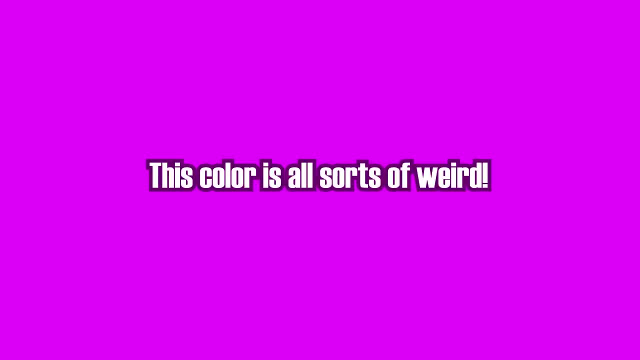 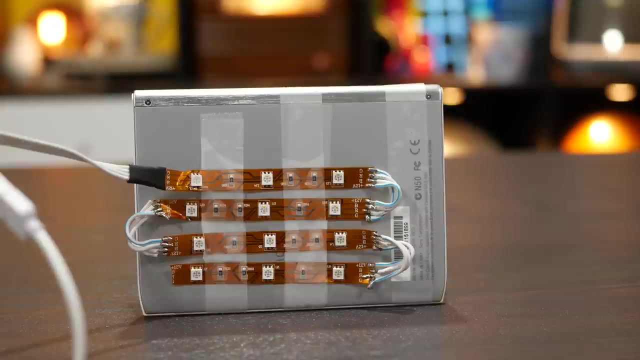 It comes from an object emitting both high and low frequencies of light, so near blue and near red, but few middle frequencies, like green. Magenta doesn't exist in the rainbow. yet there it is. Anyway, back to the tape light. These lights can make any sort of RGB combination you like, just as the sub-pixels in your monitor can. 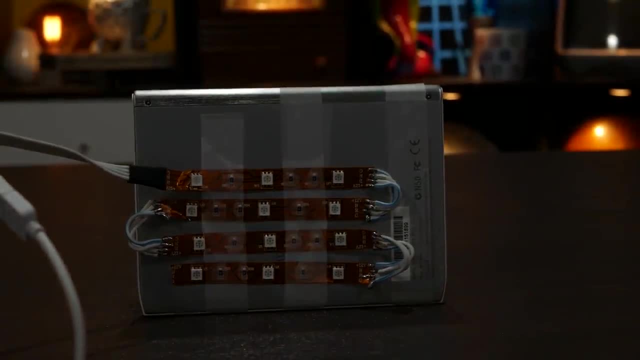 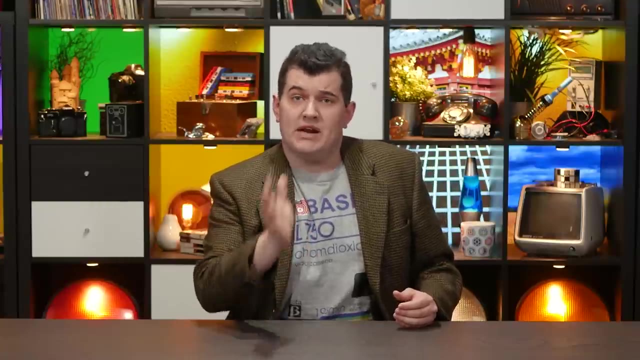 But they can't make brown. Why not? Because, again, brown light doesn't exist, There is only brown. Uh well here, how does one make brown in the RGB space? Surely it's possible. I mean, Look at all the brown. 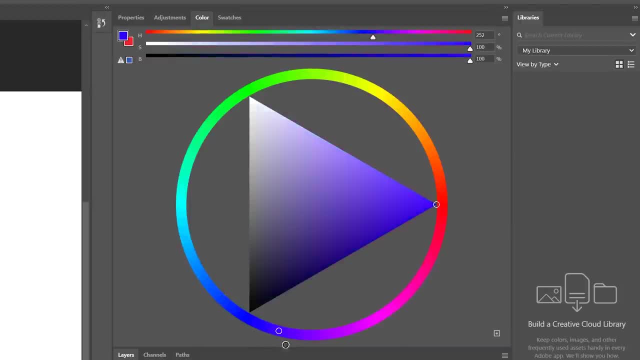 Well notice what's going on inside the triangle. This triangle represents the relationship between hue, saturation and brightness in a 2D space. If fully saturated and fully bright, we find ourselves in the right corner. All monochromatic or spectral light sources exist here. 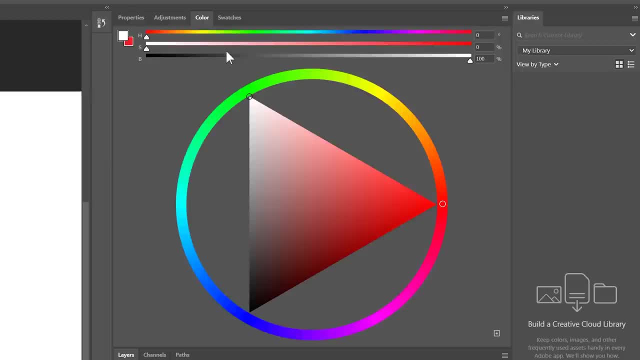 If brightness stays the same but saturation falls, we head towards the top corner and white. In an RGB space, this is accomplished by adding both blue and green to red, pushing the composite color towards white. Of note is that brightness is technically increasing, since we are adding more light. 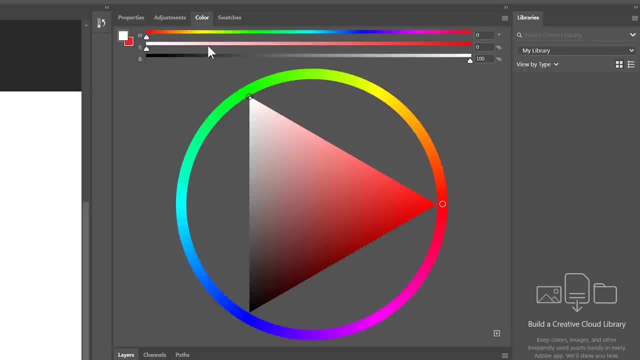 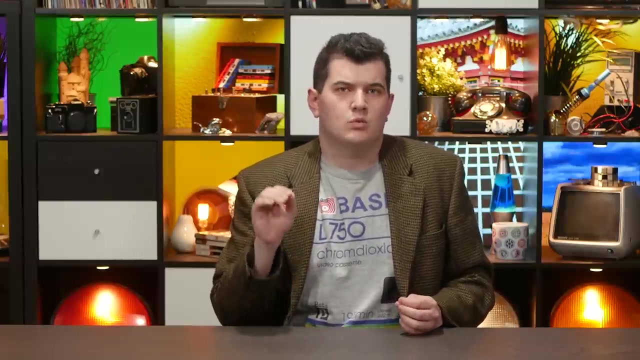 but you'll see why we don't say that shortly. As brightness decreases, we head towards the bottom corner and black In RGB. this is done simply by producing less light. As you approach no light at all, you approach black. This can be a little confusing to conceptualize because the axes are weird. 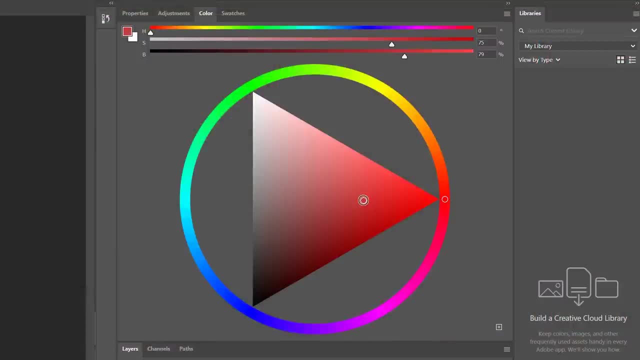 You might think saturation exists on the x-axis, going left to right, but in fact saturation remains at 100% saturation. This is because the axis is not the same as the white axis. It's a little bit confusing to conceptualize because the axes are weird. You might think saturation exists on the x-axis, going left to right, but in fact saturation remains at 100%. This is because the axis is not the same as the white axis. It's a little bit confusing to conceptualize because the axis is not the same as the white axis. 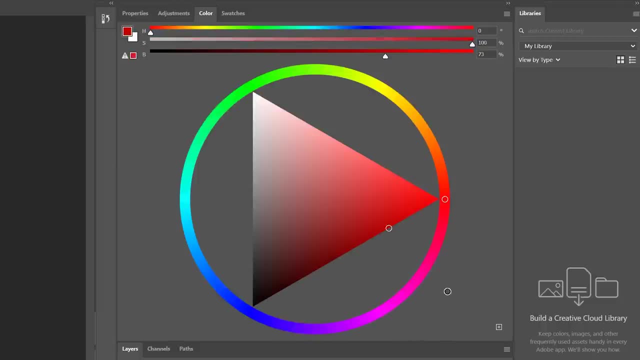 It's a little bit confusing to conceptualize, because the axis is not the same as the white axis. Only brightness varies. On the opposite edge, brightness remains at 100% as saturation changes, And on the left edge, saturation stays at zero but brightness changes and in fact, 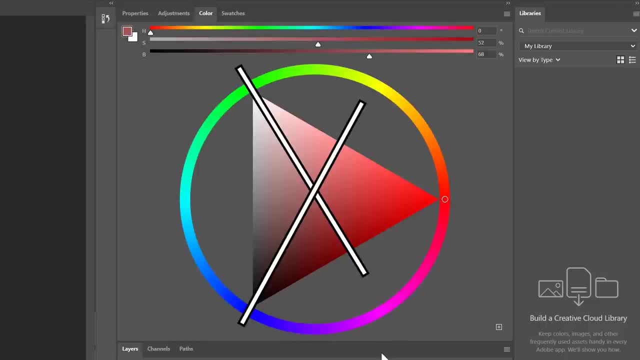 that's why this edge is simply black to white. The axes are really here, with this being the saturation axis and this being the brightness axis. It isn't really important to the point here, but it is interesting. Now, this is just one of the ways we can show a color palette. 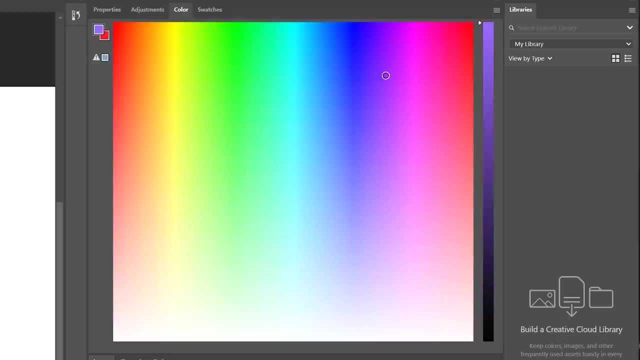 There are plenty of other options, like this one where the box contains hue and saturation and brightness is controlled via the slider on the right. Or there's also YouTube's favorite, the hue cube, but for what we're talking about here, the color wheel is best. 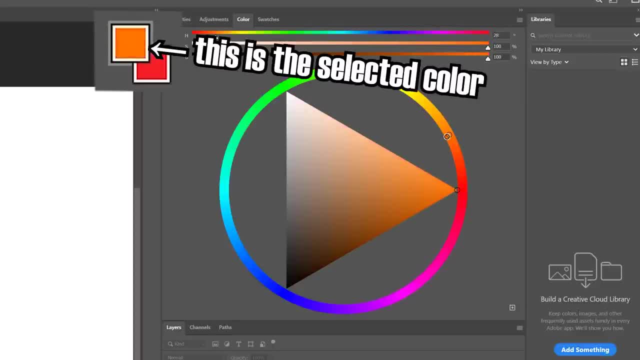 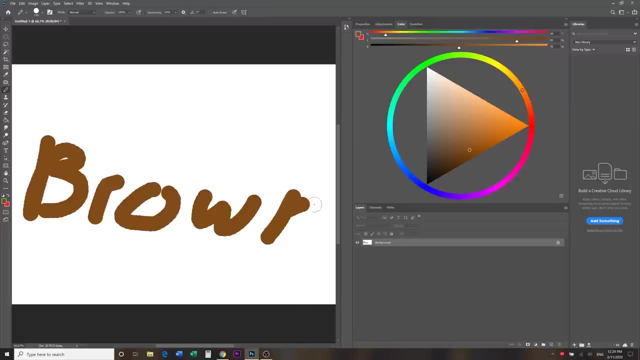 So how do we get brown out of the color wheel? Well, we're going to put our hue at something like 30 degrees and drop the brightness. That, my friends, is brown. Brown is just orange, but darker. Now. I'm sure many of you already knew this, but I am routinely fascinated by this. 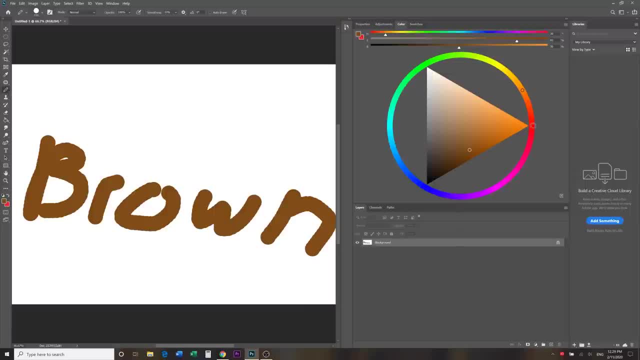 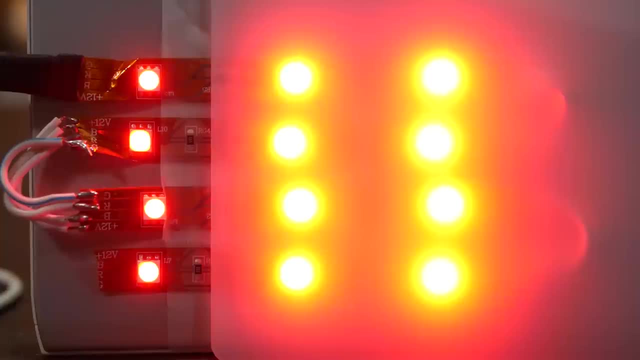 Because, again, you can't make brown light Here. let's go back to the tape light. We know that to make brown we need to make orange and darken it, So we'll make a nice orange color. Now decrease the brightness, That's still orange. 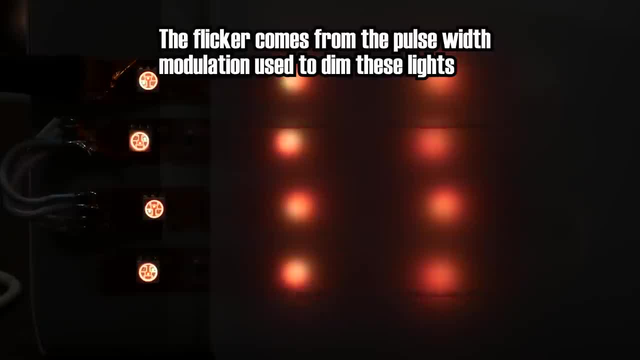 This is not brown At all. Oh, but it is. We just don't have any context to suggest that this should be brown, because you cannot create that context with a light source on its own Here. I'm going to leave you in the dark for a moment. 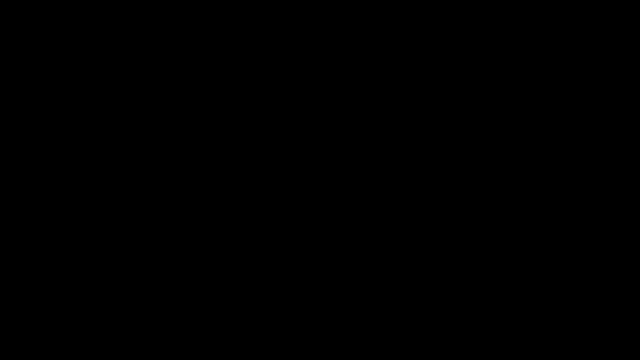 We're going to stay here for a brief period, so your eyes get used to the darkness. Yes, This sure is dark. Not a lot to see here, that's for sure. Now, this demonstration is only really going to work if you can be in a completely dark room. 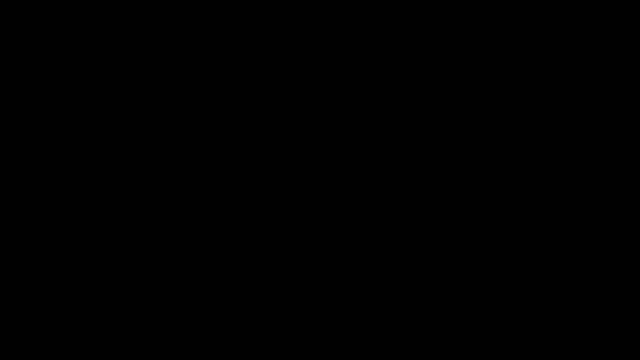 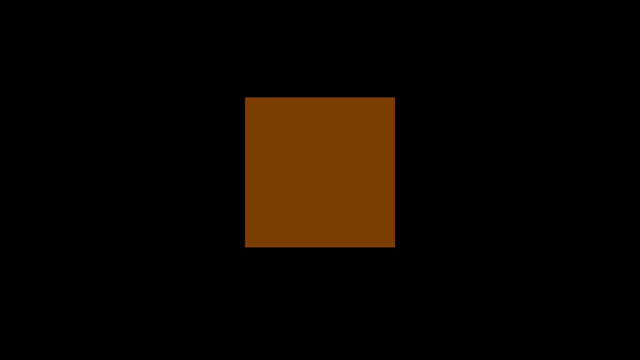 so maybe try and do that. I'll give you a second. Are you there yet? Are you in your dark place? Okay, cool. So I have brought to you a square of orange. This is a very pretty orange square, isn't it? 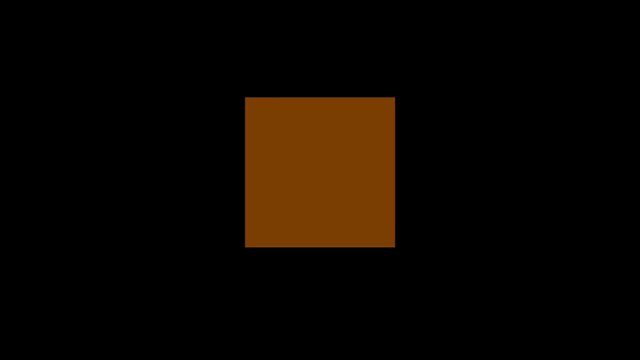 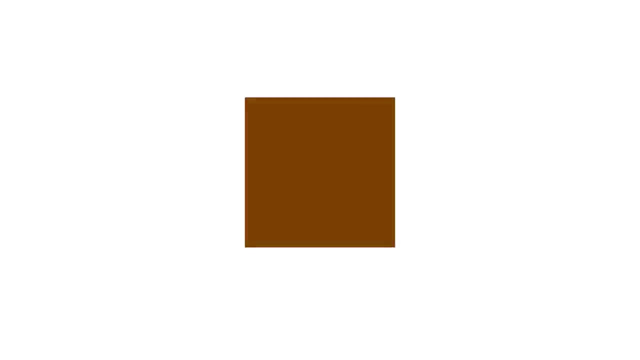 Now, it's not the brightest orange square out there, in fact I have yet to see one of those- but it sure is orange. But is it? Let's fade from black and into white? Oh no, It was brown the whole time. 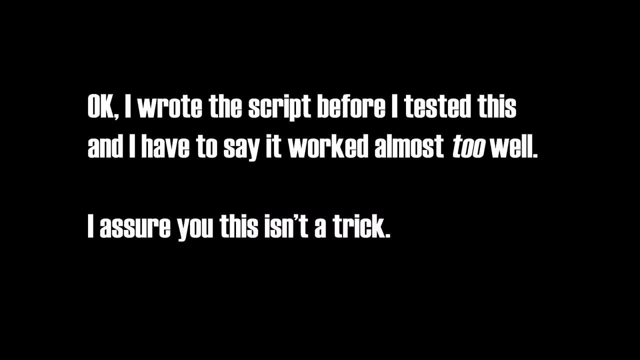 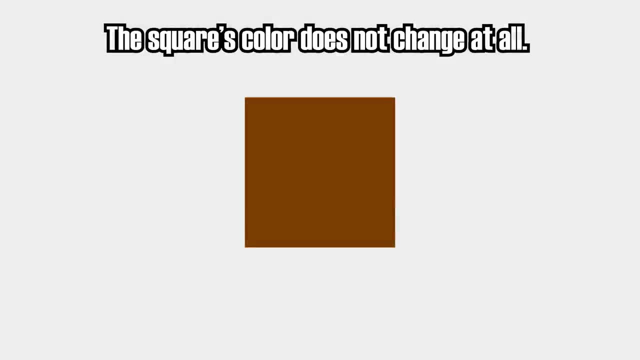 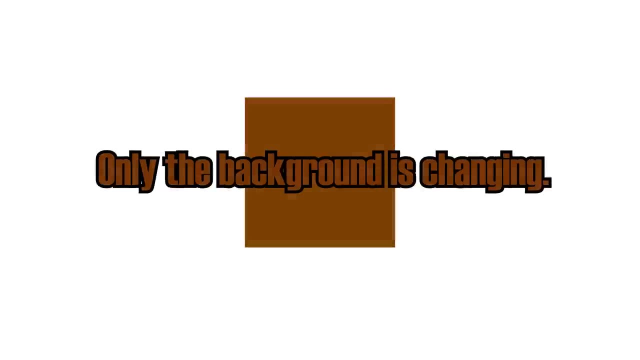 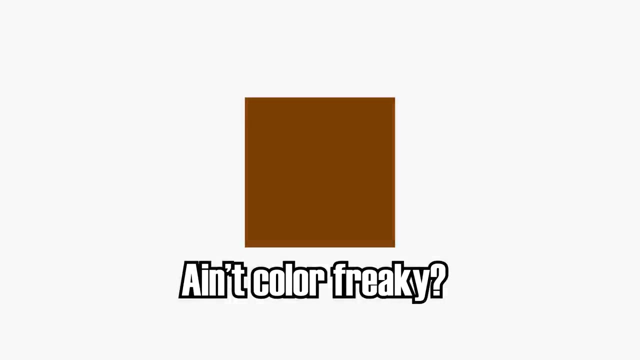 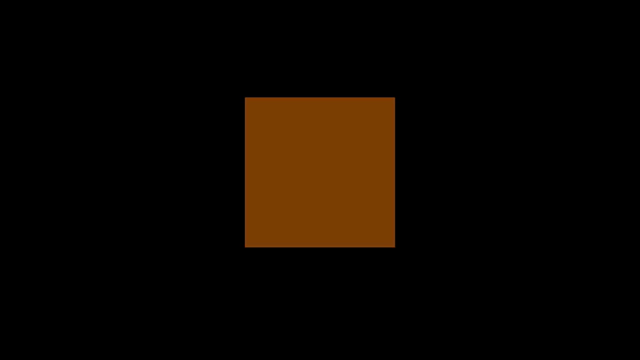 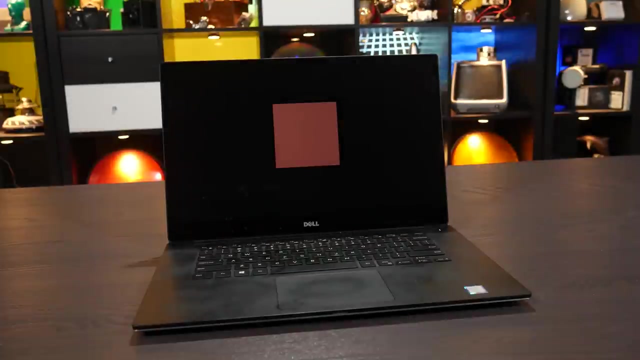 How could I have been fooled? Well, you were fooled because you didn't have any context to tell you that this color was brown. Or, if you weren't fooled, you didn't listen to me and instead left the lights on so you could see the color against the blackness of your screen. 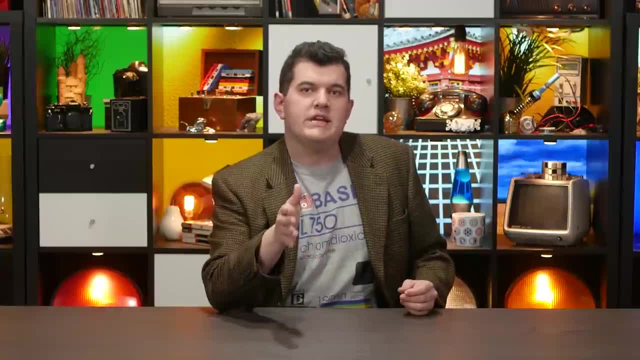 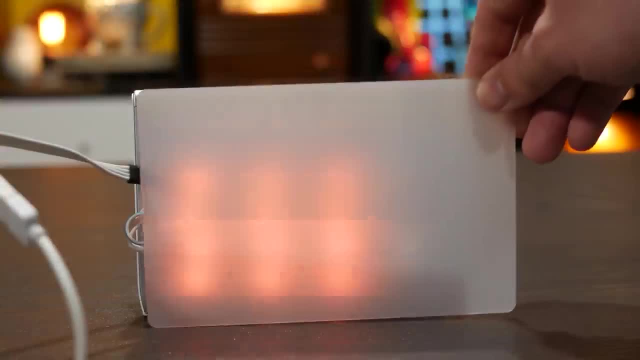 You cheater, To see brown as brown, we need to be seen very clearly And brighter things around it, And that's why you can't ever make a light source like this tape light appear brown. It produces its own light, so it will always be brighter than its surroundings. 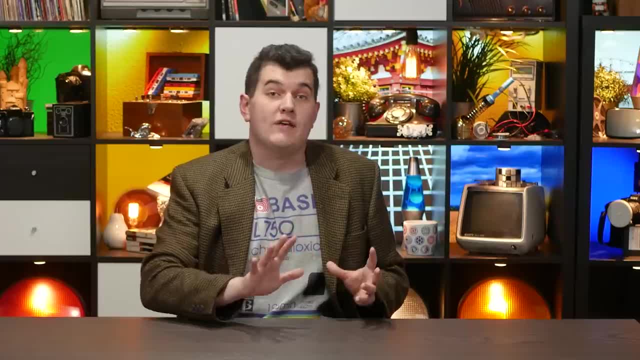 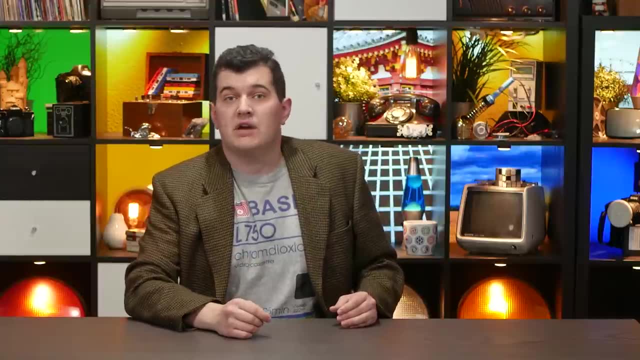 You can't use light to take brightness away. However, in the case of a monitor or television, you can control the amount of light each portion of it makes. So if you need to see a brown thing, so long as there are brighter objects on the screen, 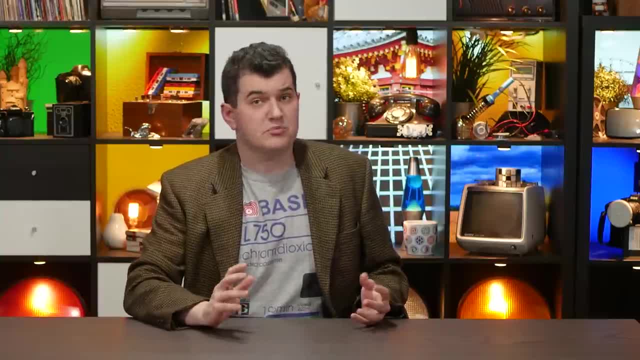 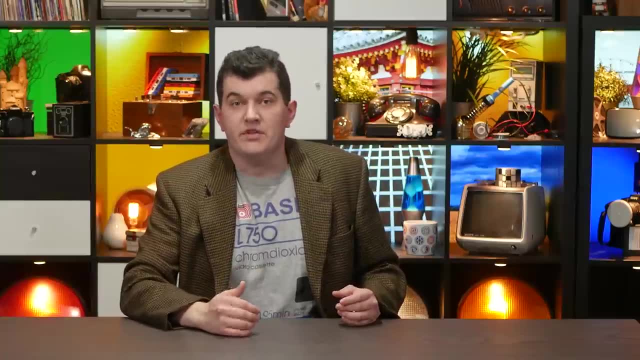 to give you context, you'll see that dimly lit orange as brown. Also of note is that with lights on in the room, the monitor is, of course, darker than its surroundings already. This is one of the reasons this demonstration might not have worked. 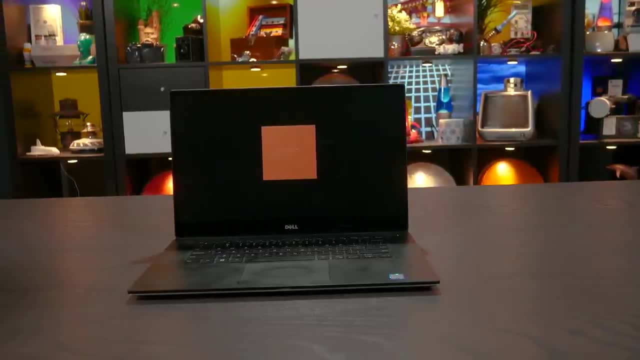 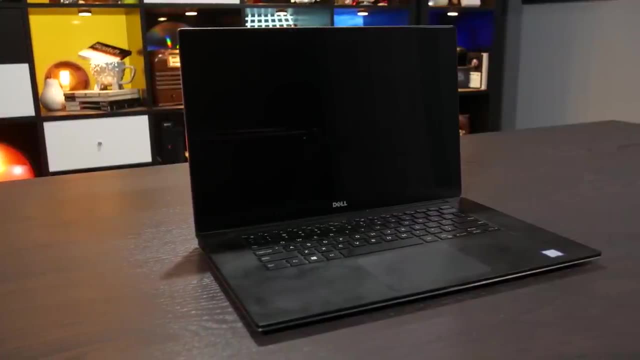 The black space around the orange square gives you the context. you need to know that it's not very bright at all, so it's brown. In fact, this is precisely the reason why your display needs to be a black void when it's not displaying anything. 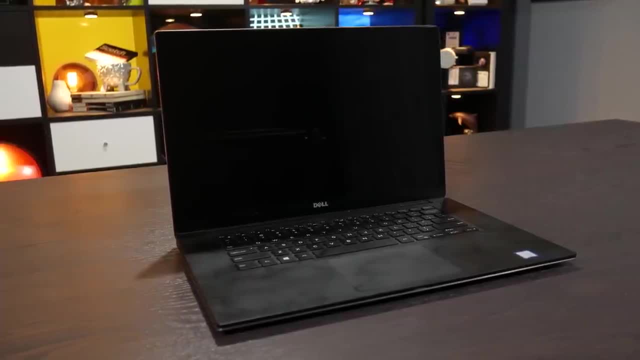 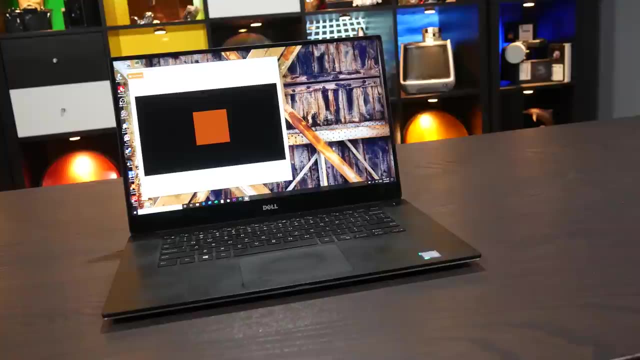 In order to see a full range of colors, you need to be able to produce darkness and lightness at the same time. The only way to do that with light by itself is to make sure the starting point is very dark, So modern displays absorb most of the light that falls on them, so they will appear black. 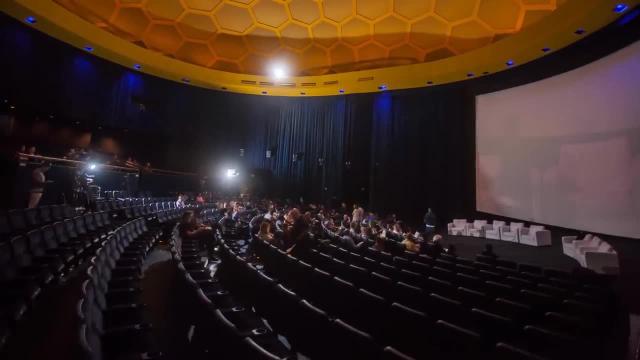 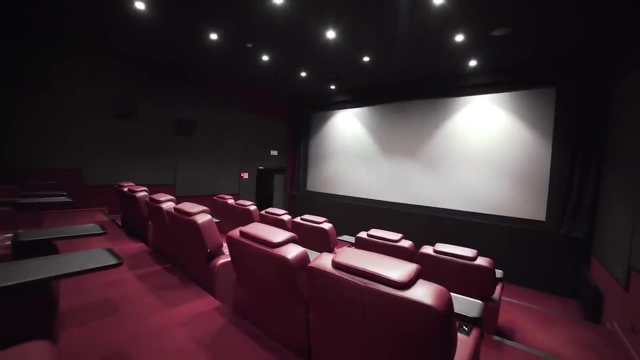 even in a well-lit space. This is also why projection systems need to be in very dark rooms. Otherwise, the screen is illuminated by incidental lighting, so the darkest color it can produce will be a gray, and the image is washed out. 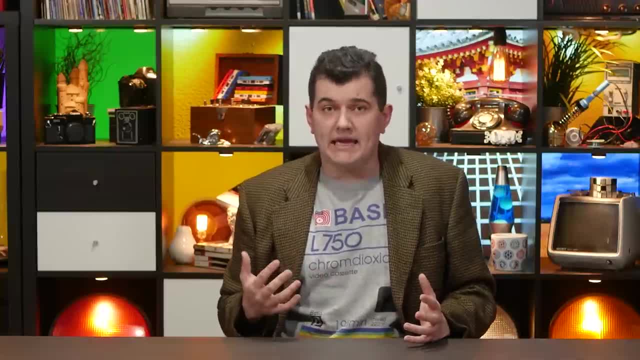 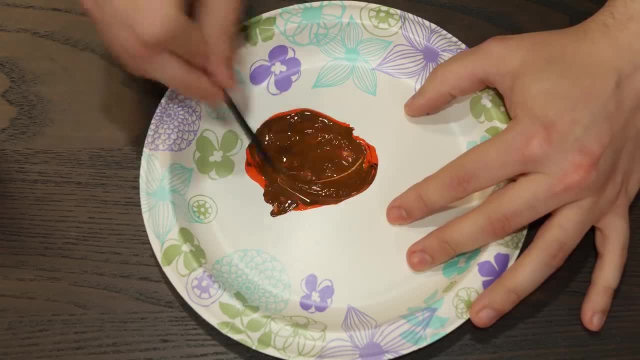 The thing is to make brown, you need to take light away. If you wanted to make brown using pigments, you'd start with orange and add black, And in fact, you can even see this going on in the color wheel. While this is, of course, representing color in the context of light, you can also think: 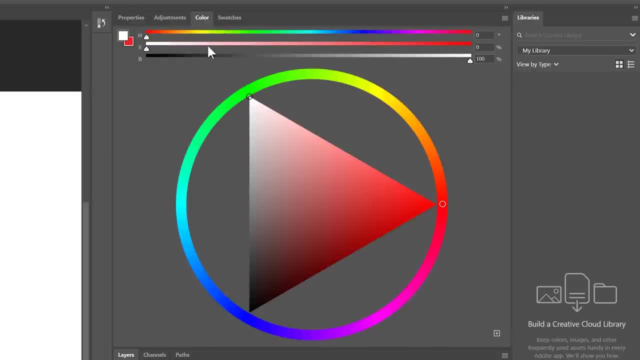 of this as the result of mixing paints together. Up here is purely white paint, Down here is purely black paint And over to the right is a paint of perfect hue. Mix them together and you get what's going on inside the triangle. Objects in the real world that are brown are like light. Like an orange mixed with black. The light they reflect into your eyes is similar in wavelength to an orange, but there's not a lot of that light. It's pretty dark, And we just happen to call that resulting color brown. Side note: brown is also fascinating to me because it's arguably a human construct. 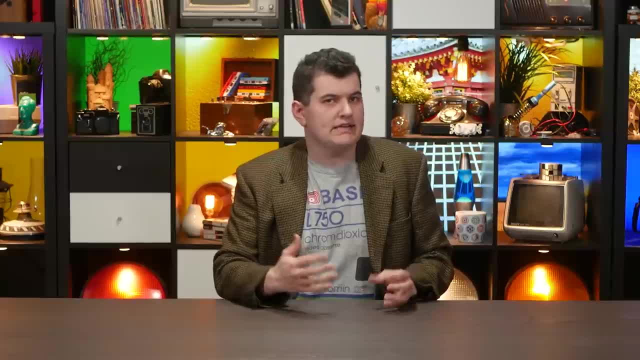 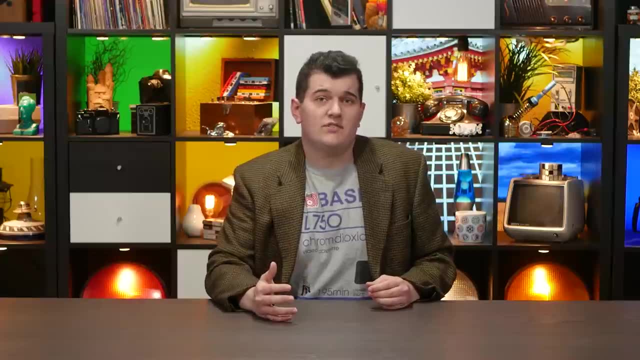 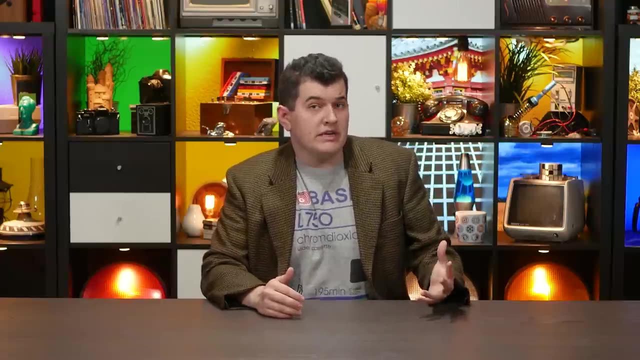 Perhaps you've heard about how languages evolved to describe color in categories. Some languages have fewer categories of color than others, and anthropologists have discovered that as languages evolved, they tended to build upon these categorizations in the same predictable order. For instance, languages with only three categories of color would almost always contain white. 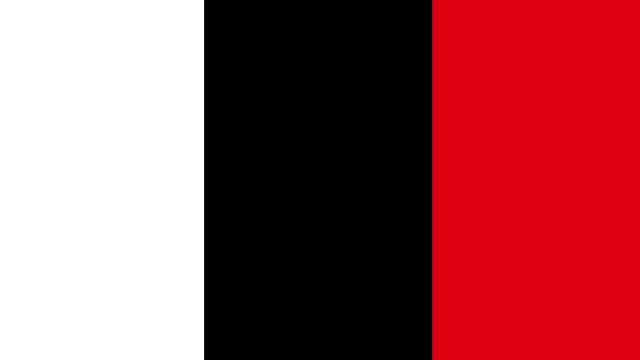 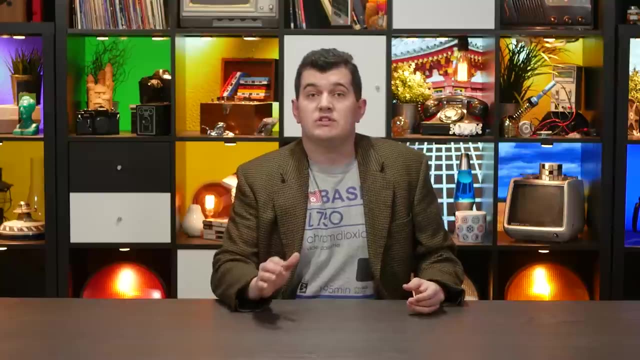 black or their stand-ins, light and dark and red In these languages, things like blue, green, yellow. they just don't have words for them and they're not distinct. Languages with six categories, like mantra and Chinese, contain white, black, red, yellow. 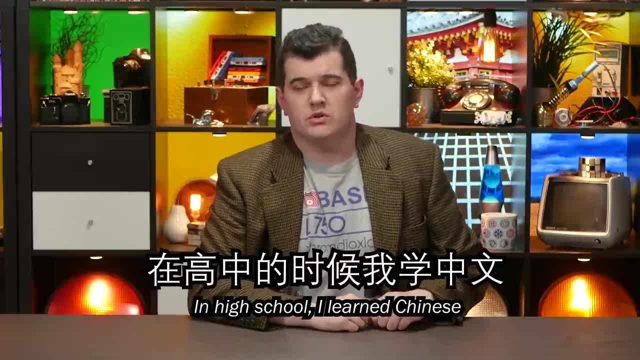 green and blue Side side note: 在高中的时候我说在高中的时候我说在高中的时候我说: When we were learning colors as you do, we learned. 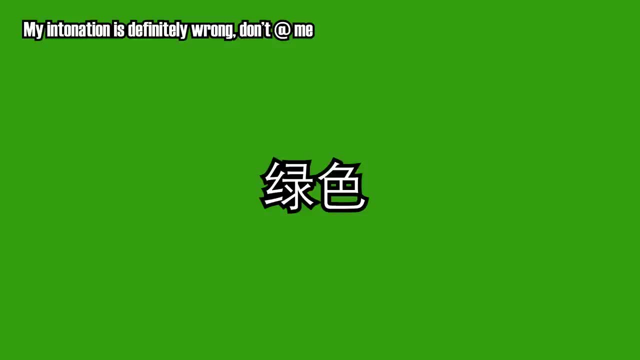 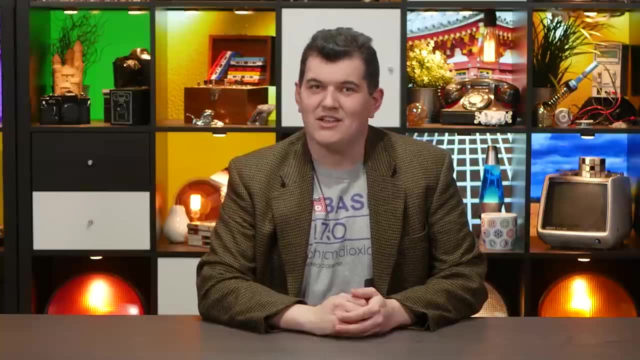 白色, 黑色, 红色, 黄色, 绿色 and 蓝色. Then our teacher asked us: What do you think brown is? And I blurted out because I was a smartass and thought it would be clever. 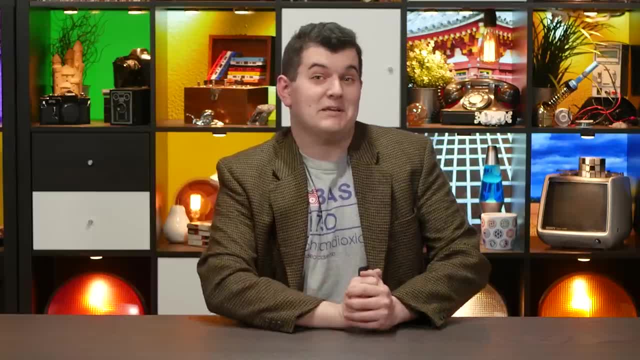 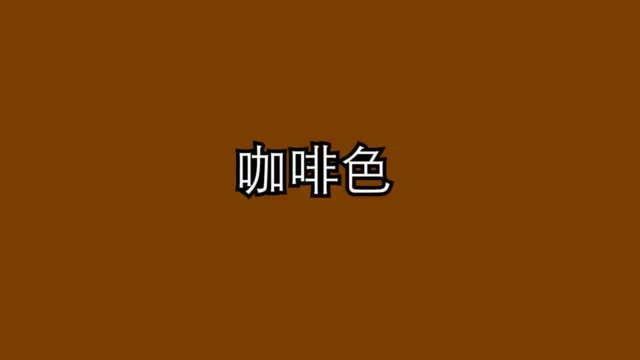 What is it? 咖啡色? And my teacher's eyes lit up because it is Now to be fair. that technically means the color of coffee, And there is a separate word for brown, 棕色. 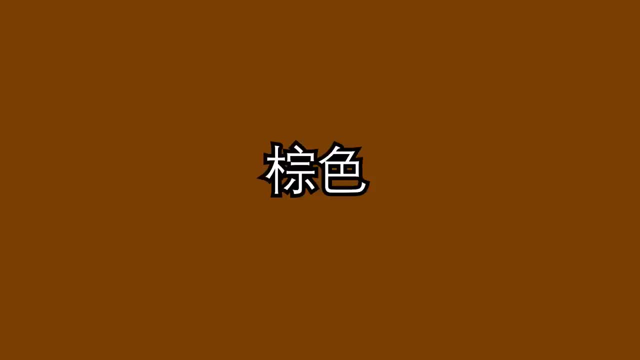 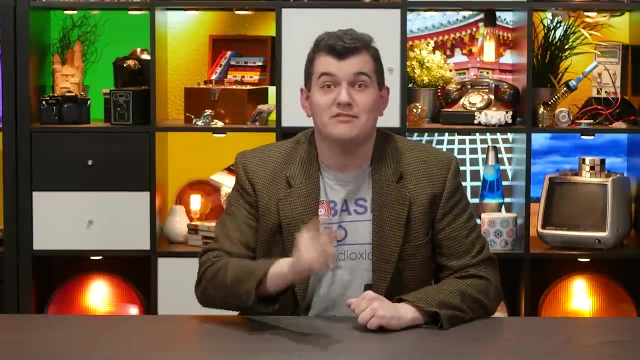 However, we used 咖啡色 more frequently than we did in the past, More frequently in class at least. so there you go. I can now officially say that I have used my very, very rudimentary knowledge of Chinese in my professional life. 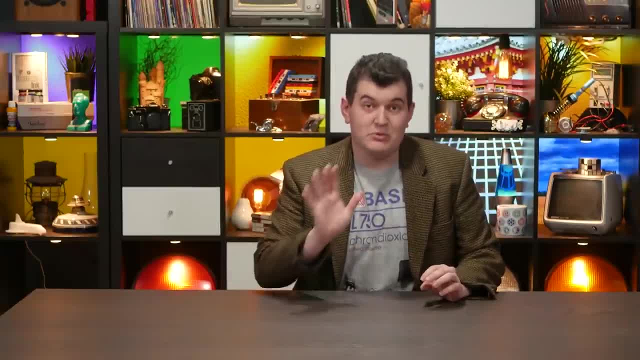 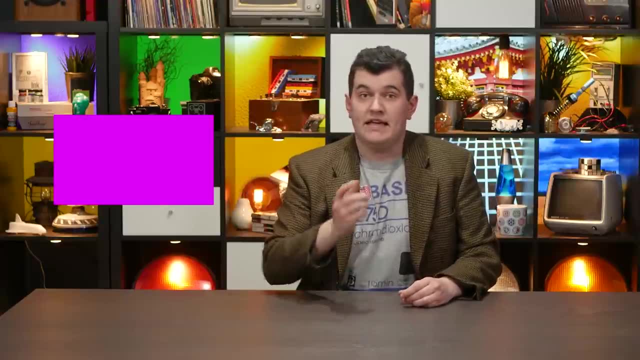 Huzzah. Anyway, to get us back on target, the point I'm making here is that we only recognize colors as distinct after we've decided that's a distinct color and we give it a name. Even in English, orange didn't become a color until we stole that word from the fruit. 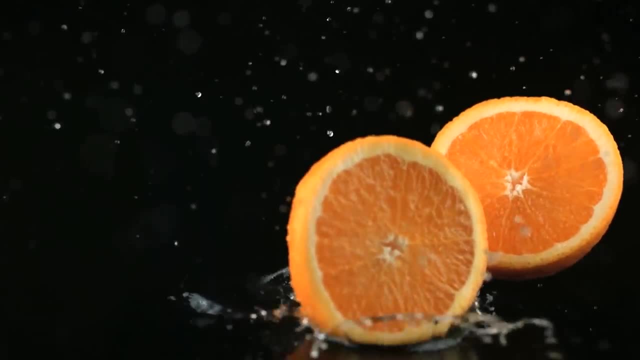 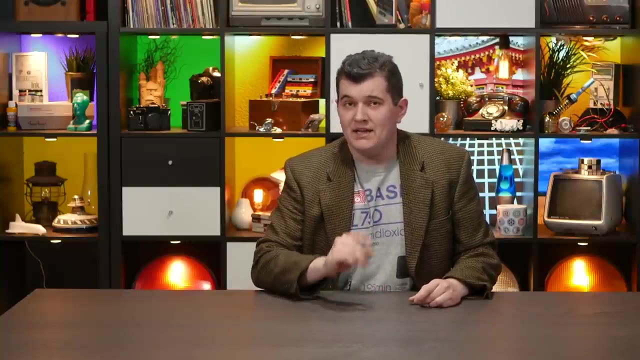 Prior to then, it was either yellow or red, Or yellow-red, Or maybe red-yellow Rello, Hmm, And I think brown is definitely one of these late colors. Why, Well, let's hop on board the color wheel one more time. 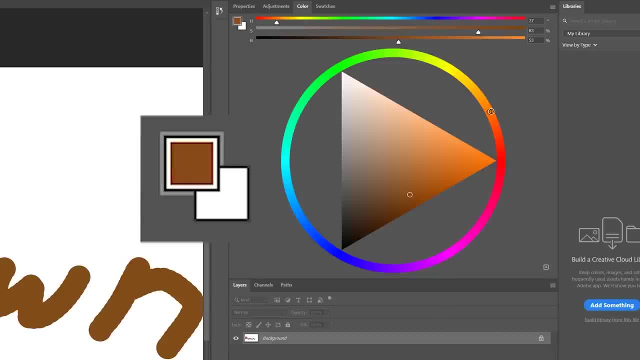 Right here is a nice sturdy brown. Clearly that's brown, But look what happens when I change the hue. As we head into yellow, that becomes- oh, I don't know- a pukey green, Maybe tan. We move into green and that's just a dark green. 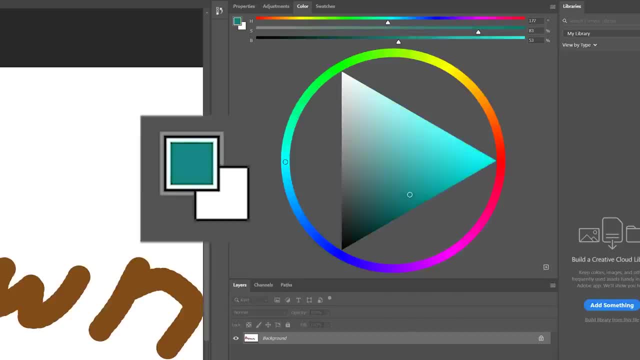 As we move into cyan, we get a dark green, We get what you might call a teal, but everything from there on out is just dark, whatever Dark, blue, Dark purple, Dark red. But when we get back to orange, that's not dark orange, it's brown. 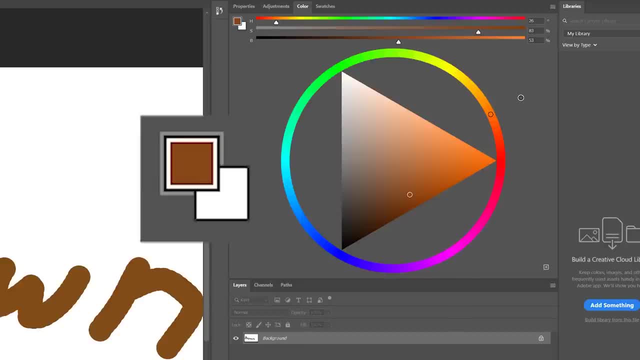 The color is clearly its own color, But why? Why isn't it a dark orange? Well, because we've named it brown, And the mere act of doing that causes it to become a distinct color in our mind's eye. That's pretty neat and weird stuff, isn't it? 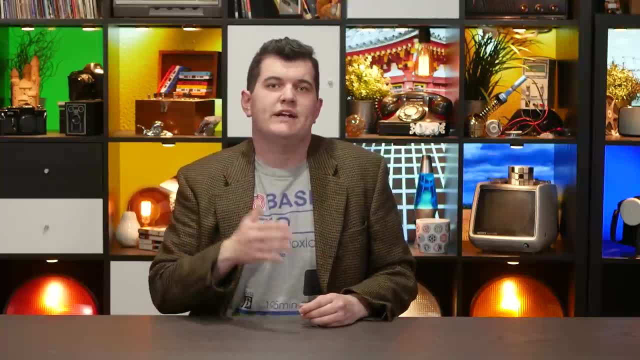 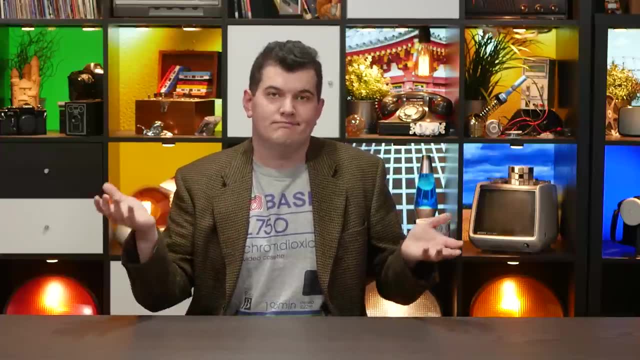 Brown serves as a fantastic example of that. Brown serves as a fantastic example of that. Brown serves as a fantastic example of the difference between creating color with pigments and creating color with light. Objects in the real world are lit by the sun or maybe a lightbulb, and what we see is the. 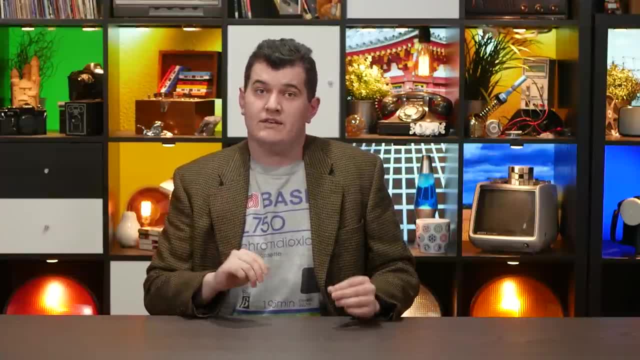 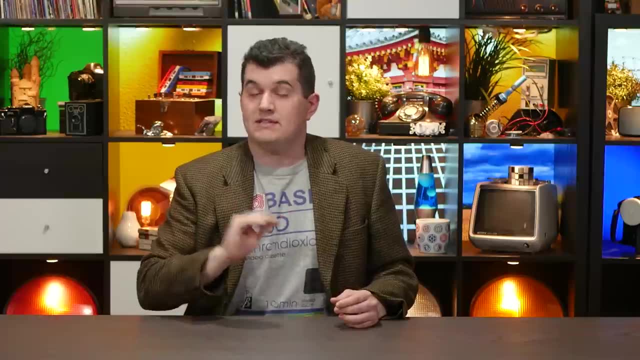 light reflected off of them. If they reflect a lot of that light, they'll appear white. If they absorb a lot of that light, they'll appear black, And if they absorb only some frequencies of light and reflect others, they'll appear as whatever color they reflect the most. 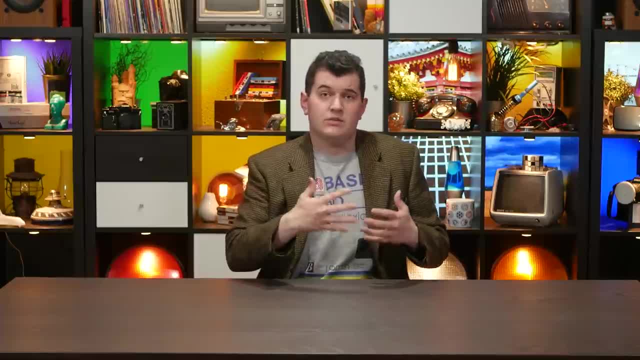 But describing it that way is incomplete. It's not just the prevailing wavelength that's important. It's not just the prevailing wavelength that's important. It's not just the prevailing wavelength that creates the color, That defines the hue. Again, that's the circle. 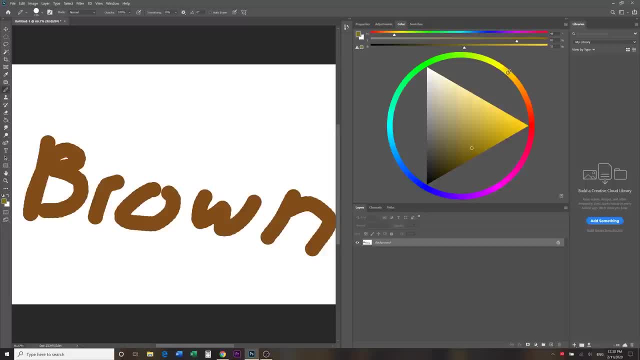 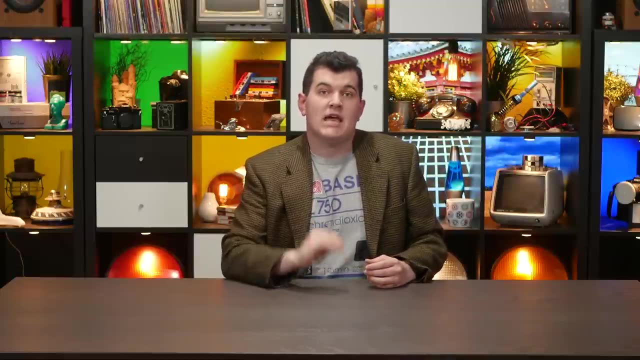 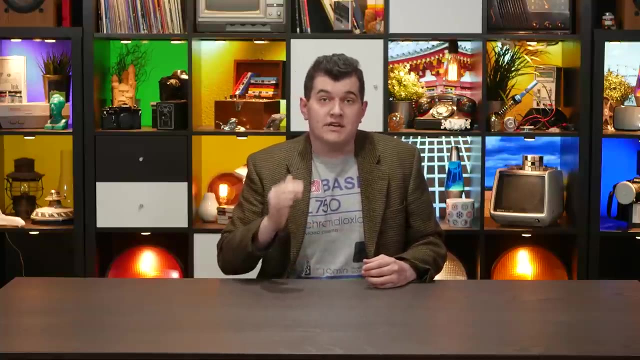 Hue is only one third of color. Hue, saturation and brightness all work together to create the colors we see In the realm of pigment or real-world objects. brightness describes how much light is reflected back. hue describes which, if any wavelengths stand out to give it color, and saturation. 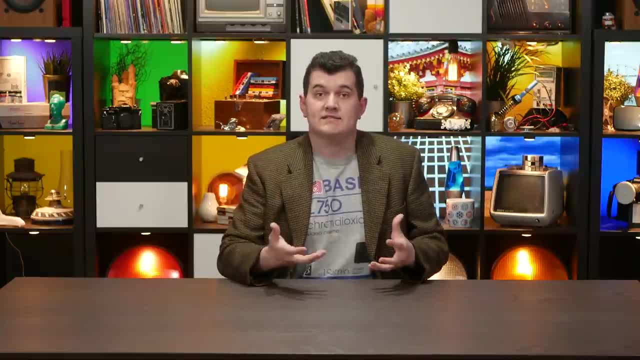 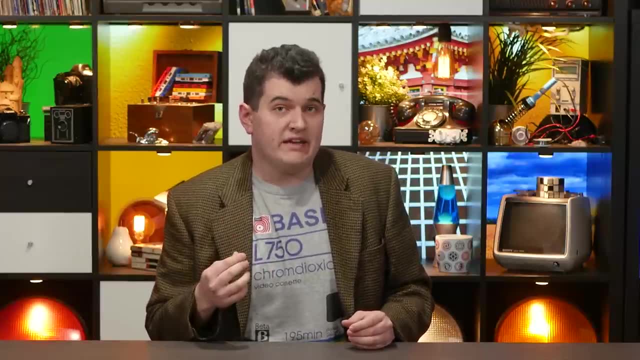 describes how much that wavelength stands out or how intense the color appears. And the thing is: in the real world we don't see that. In the real world we always start with light and the objects around us take it away. This is called subtractive color. If we use paints well, a white paint reflects pretty much all of the light that hits it back, and roughly equally. A black paint absorbs most of the light that hits it again equally. And a colored paint absorbs most light, but not certain wavelengths. 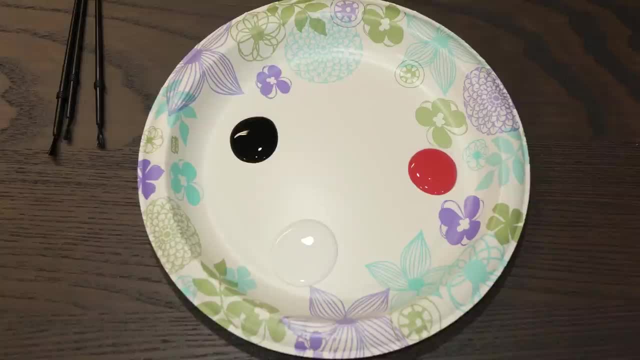 In the case of red paint, it reflects red quite well. In this scenario, the red paint is our hue. Red paint alone is fully saturated. It's saturated and fully bright. Add some white paint to it and you decrease the saturation, because now the reflected 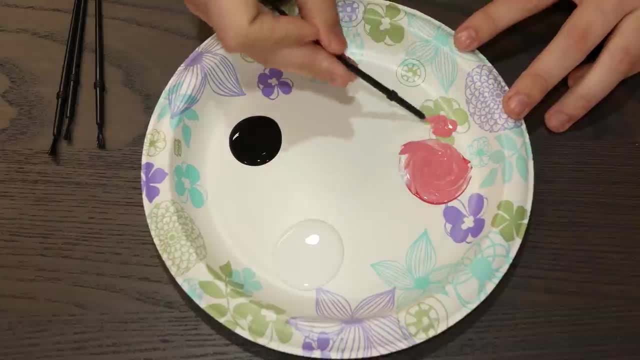 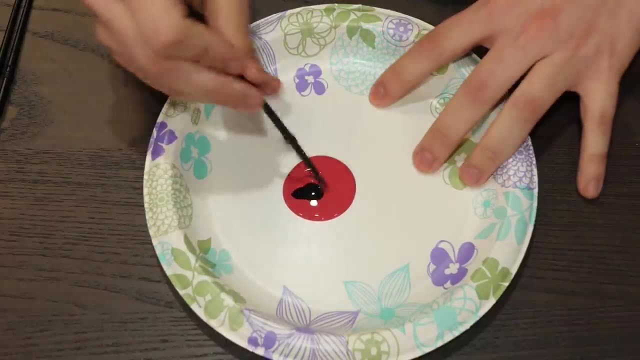 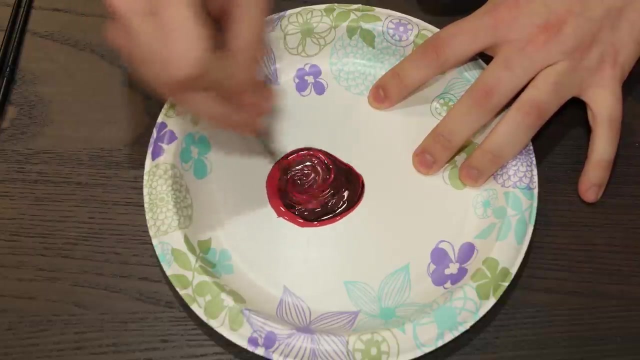 light is not purely red. Other wavelengths are now visible, though red remains prominent. Mixing in black paint with red decreases the brightness because it lowers the overall amount of light being reflected back. However, because black paint absorbs all wavelengths roughly equally the light being reflected 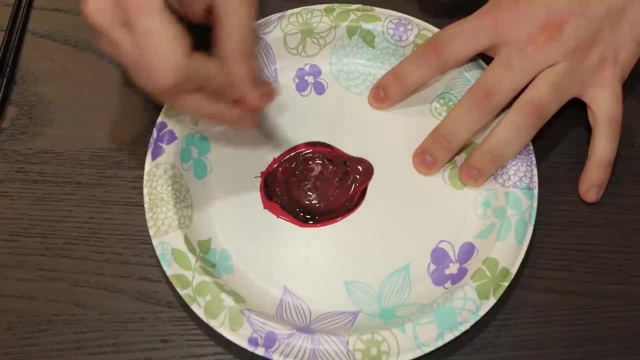 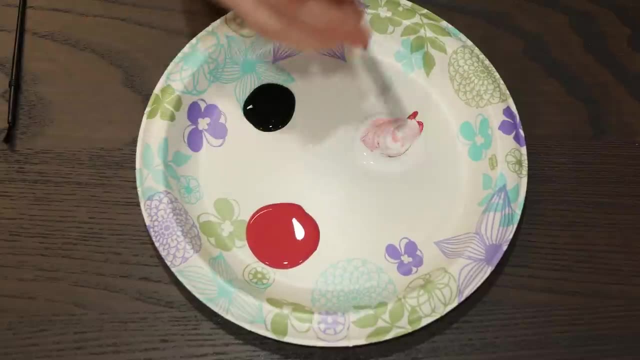 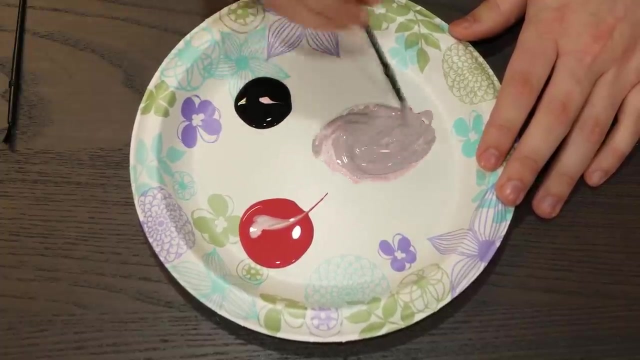 back is still purely red. there's just less of it. So this mixture is fully saturated, but less bright. You can create any brightness and saturation combo you like simply by altering the ratio of white, red and black paint. The hue, however, will always remain red or roughly zero degrees on the hue circle. 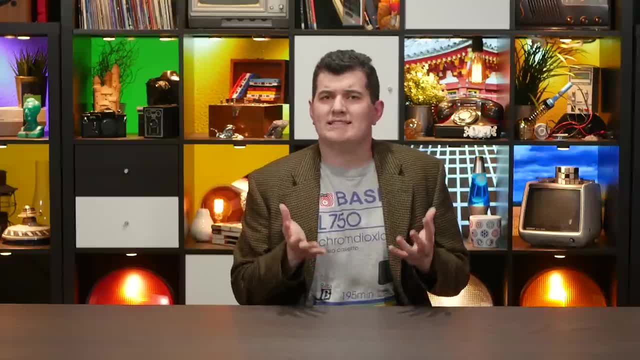 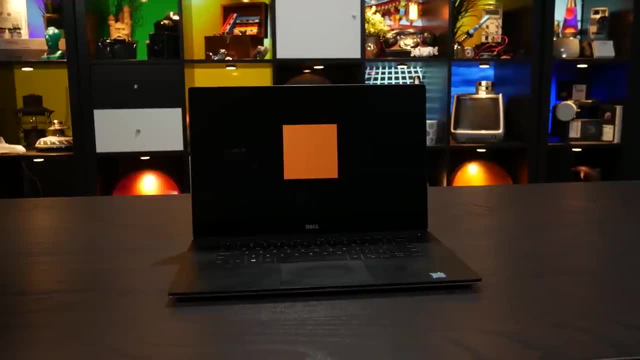 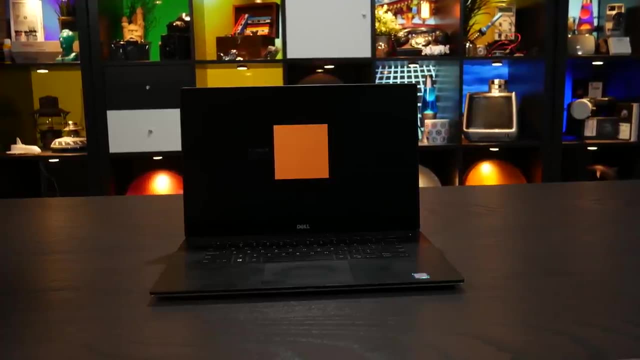 But when we use light to create an image, this is sorta turned on its head. A display creates its own light usually, and this is why the primary colors are red, green and blue. We sometimes call this additive color. We are starting with no light and need to add light to create what is seen. 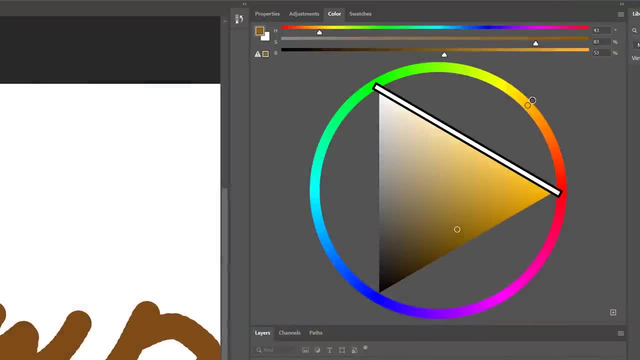 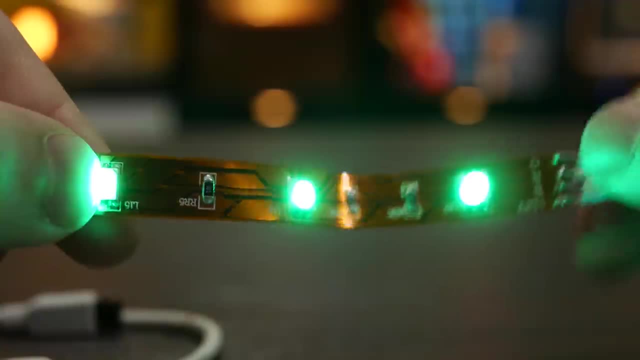 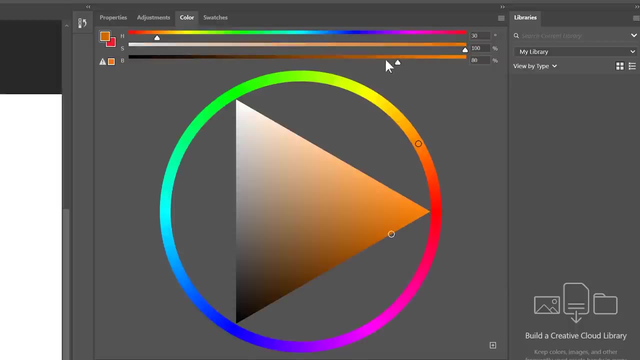 And in the weird world of RGB, creating colors anywhere below this line requires lowering brightness or taking away light. But we can't actually take away light, We can only produce less of it. And that's what's so interesting about brown. Even here on the color wheel, with orange selected, it's kinda hard, at least to me. 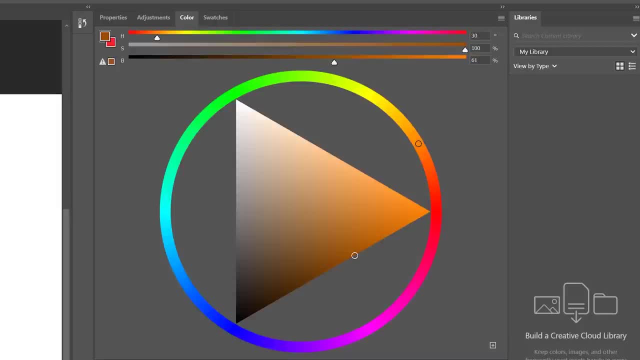 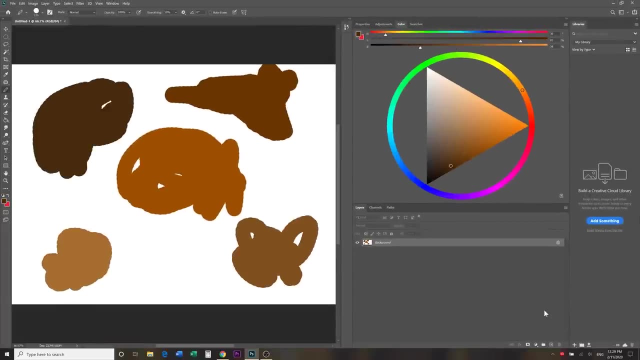 to see the space in the triangle. It just looks like a whole bunch of different shades of orange, But indeed those darker shades are very much what we call brown. It's an orangish wavelength of light, but not a lot of it. 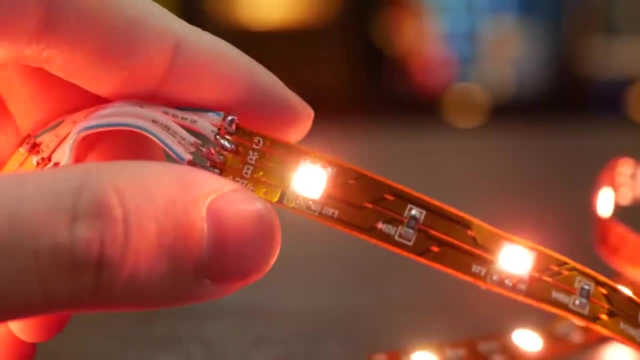 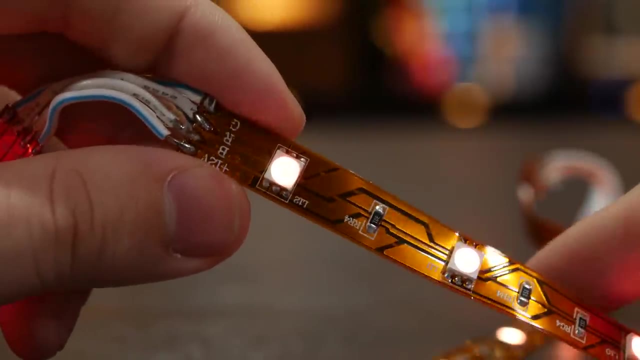 With something like an LED tape light or really any RGB light source on its own, you can't produce a color that looks like brown, because any attempt to do so will just end up looking like orange, And the reason why is pretty simple: All light sources brighten what's around them. 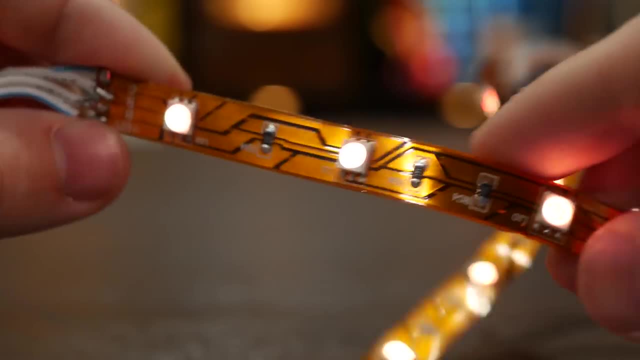 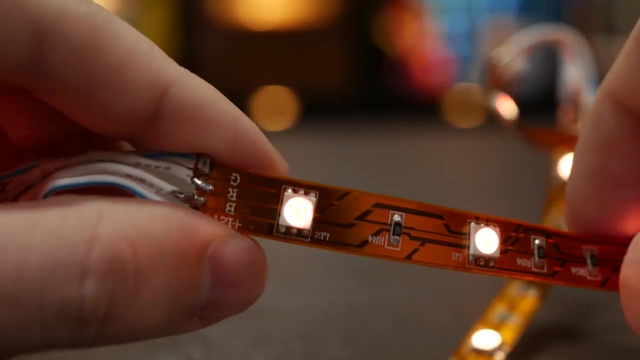 There's no equivalent of a black pigment in the realm of light. There's just… less light, And in order for that to be perceived as a dark color, you need to have some sort of context. You get gobs of that when looking at an image produced on a display, but you get none at 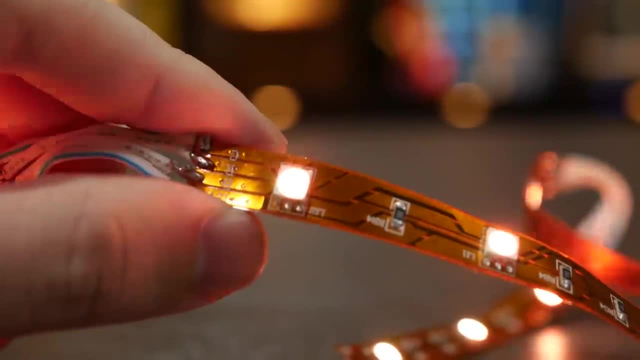 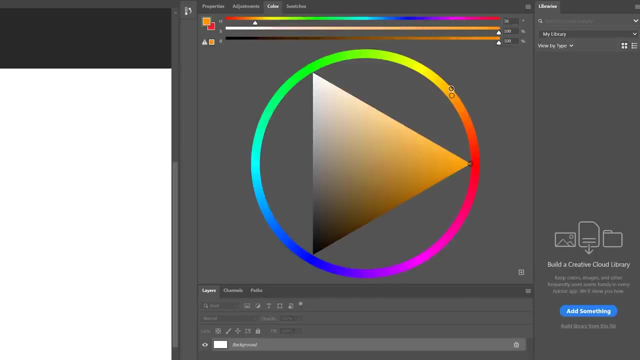 all from a simple light source existing in the real world. With an RGB light, you're limited to colors that exist on this line. You can either have a pure hue, which, incidentally, is why your RGB gaming rig tends to have a light source that's not a light source. 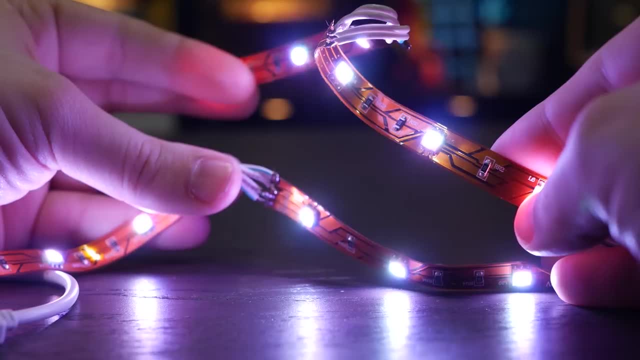 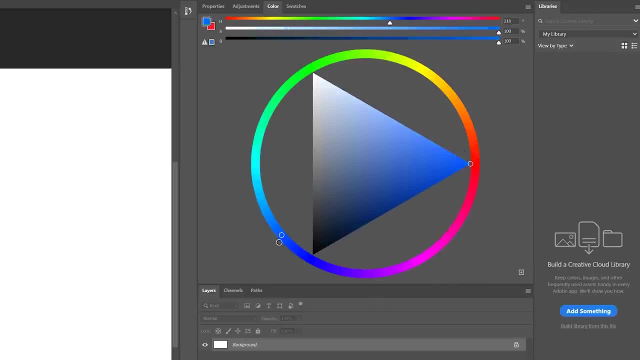 It tends to just cycle between blue, cyan, green, yellow, red, magenta and blue again. Or you can decrease saturation and approach white, But you can't venture away from this line. I mean you can, but a dimmer light without context is still just a light. 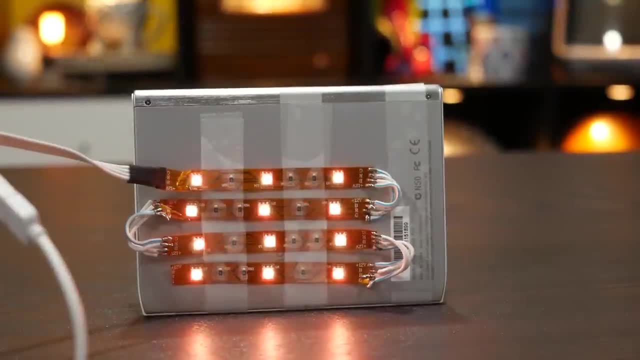 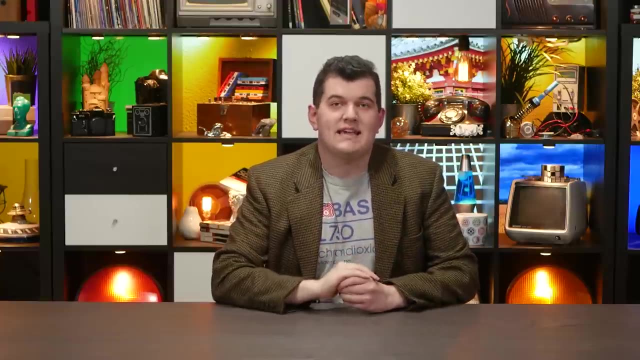 And our brains simply won't see that, as in the center of the triangle, unless we have other, brighter things to see too. I hope you enjoyed this look into the color brown. Brown is, and I am not kidding you, my favorite color. 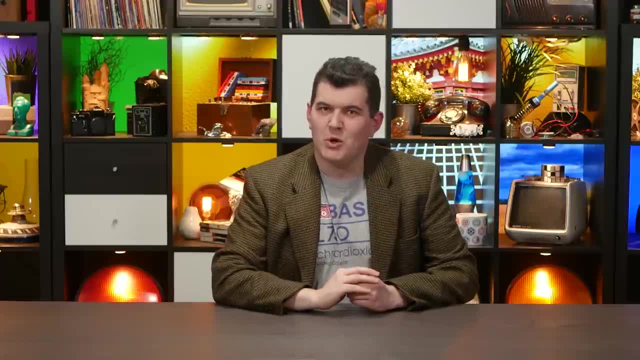 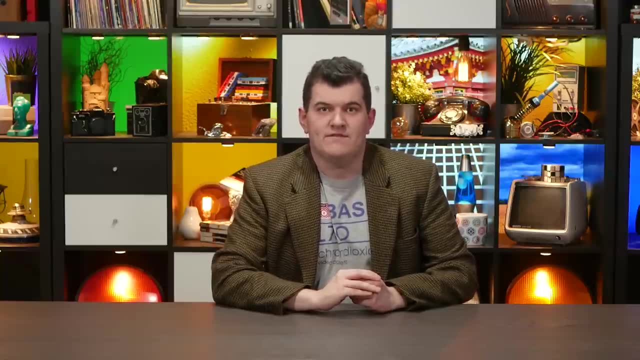 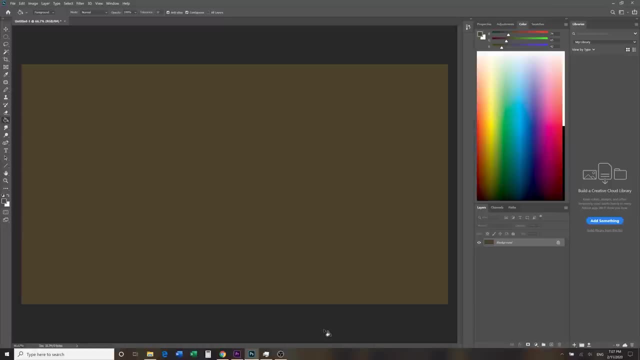 Sometimes I wish we could just get a 70s appreciation movement going, because boy was that a good time to be a fan of brown. Nowadays nobody seems to like the color brown- Sad face. Now, to be fair, the world's ugliest color- that's Pantone 448C- is a brown. 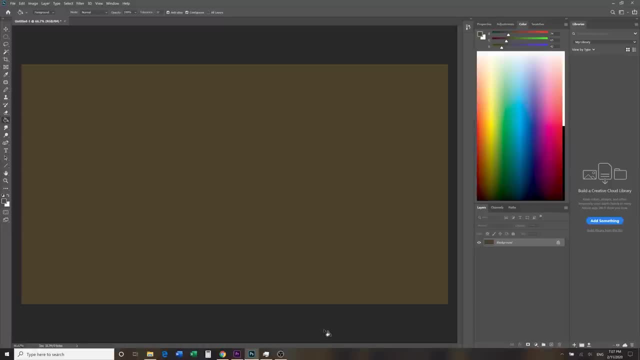 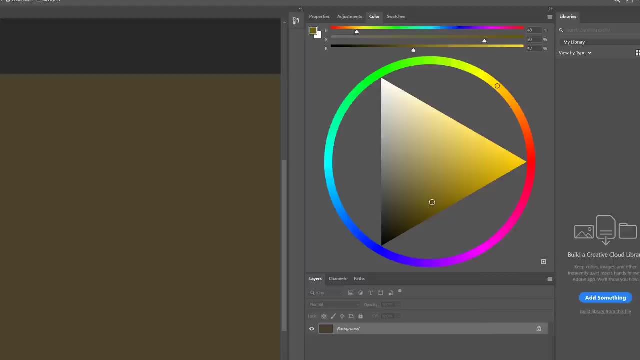 But I mean, that's not fair to brown. Not all browns are that gross looking They can be. Just slide the hue over here and you're getting a good bit of yellow in there, which somehow seems to make the brown look almost greenish. 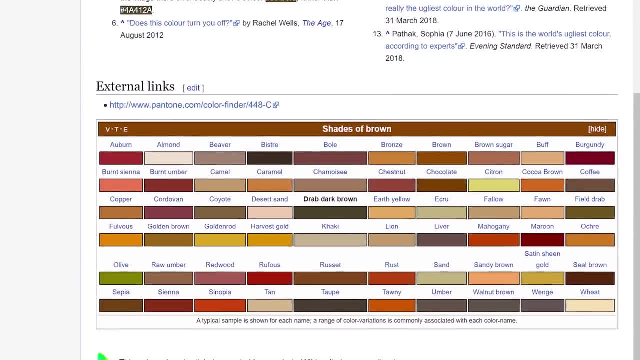 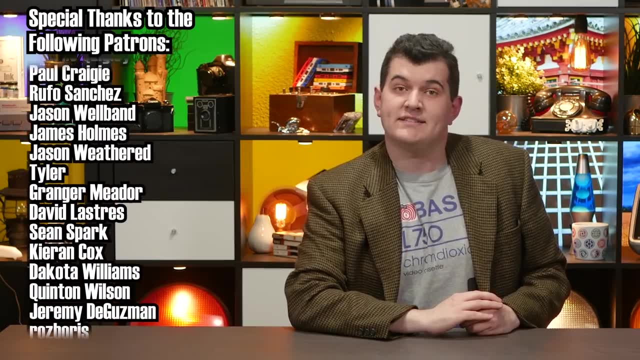 But Just look at all these other great browns. Those are some good browns. Are you wondering why I've made a video on brown? Well, the more good sounding answer is that I wanted to share with you more of the weirdness.